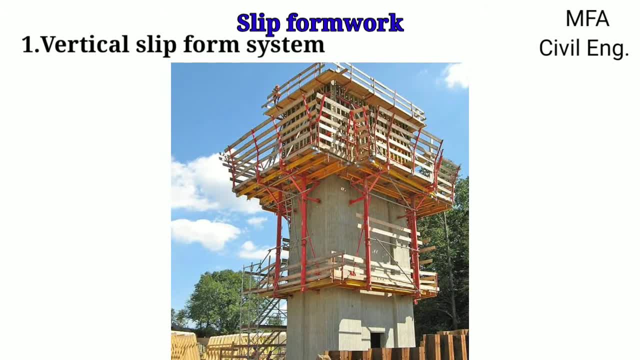 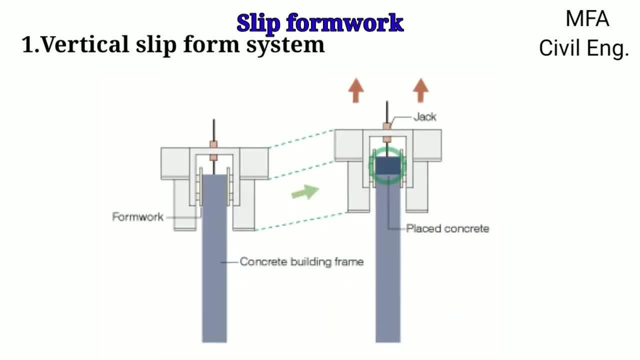 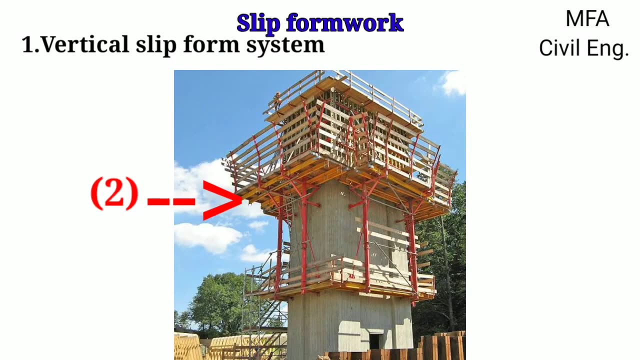 the slave form. The main important advantage of the vertical slave form is that no need to build and dismantle the excessive scaffolding. Vertical slave form has the two limitations: like the wall has to be vertical, the wall has to trace an unchanging horizontal projection. in cantilever jump form system, the 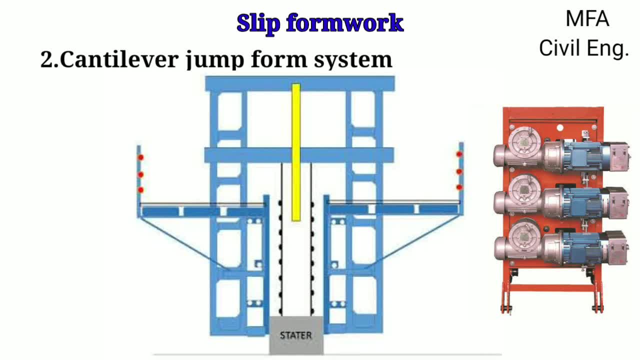 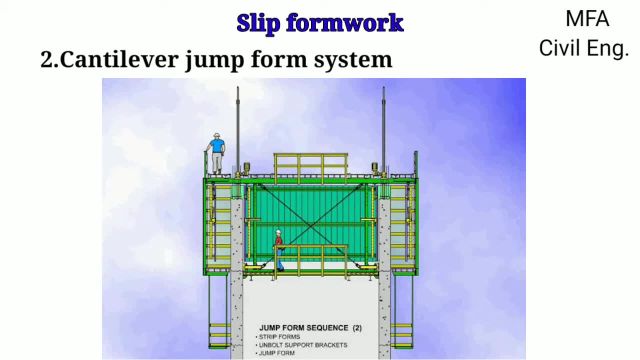 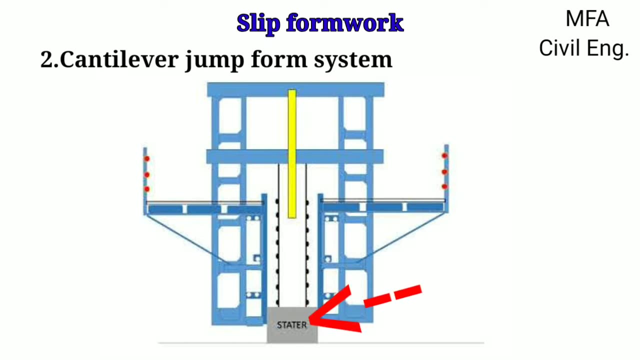 lifting device is simultaneously driven by the electric motor. the main advantage of the system is that the climbers are independent of the crane and attached to the large area form of at the story height. in the system, shuttering can be fixed to the already completed part of the structures. 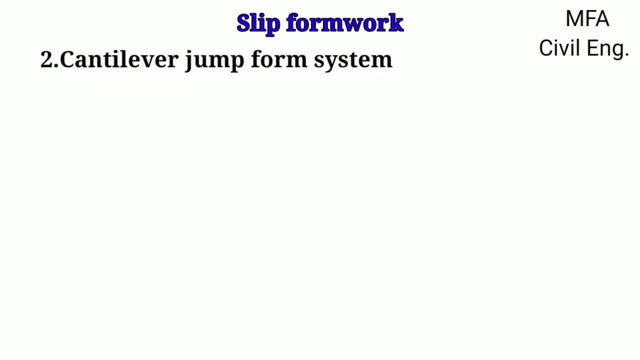 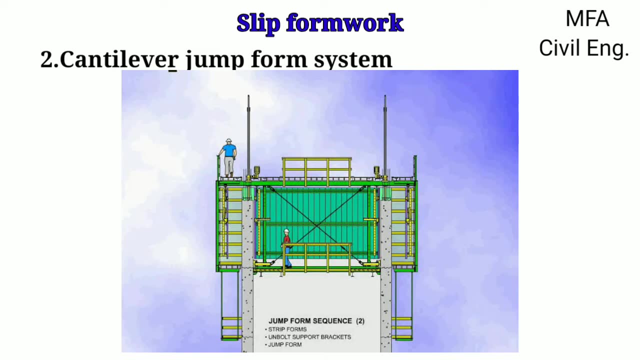 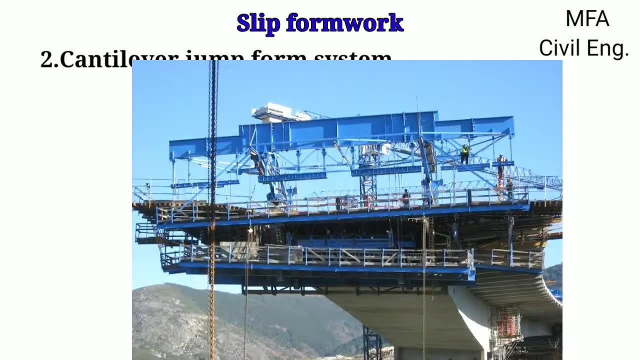 between the individual level of the climber. cantilever jump form system give the maximum safety. it provide a complete self-climbing formwork system which is independent of the crane of a wall column supports and the floors barrier. for precast floors, cantilever supports are easy. 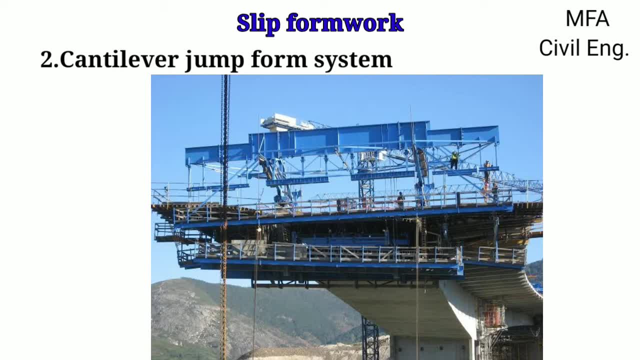 to install and built-in element can be placed accurately. upper gutter work system provide a work deck for the material handling and concreting. it is fully enclosed system which provide to proceed the work of the concreting safely and with a great comfort and protect from the weather. in this system, any building and dismantling. 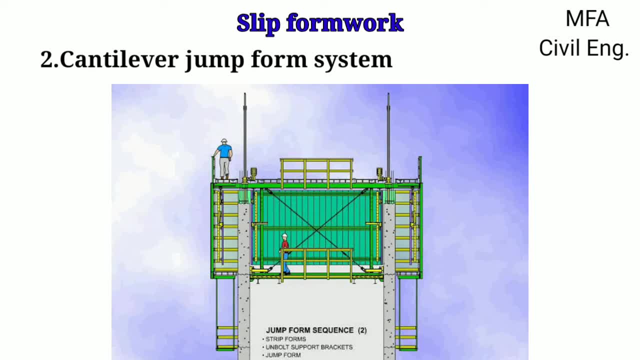 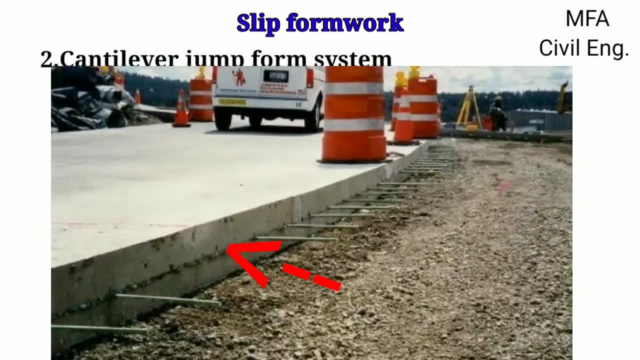 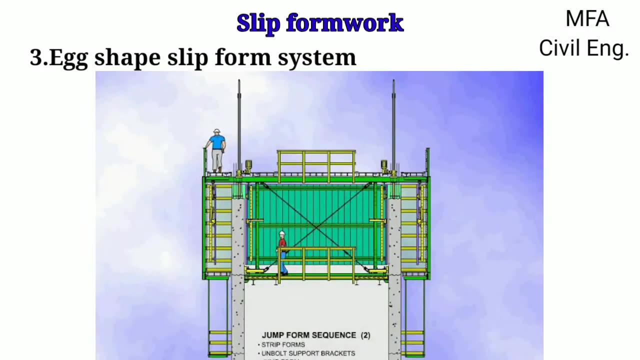 work of the excessive scaffolding is completely eliminated. the great advantage of a sleeve form construction is that it provide a rigid cast structures which is free from the ties and cold joint. the egg shape sleeve form system is based on the jump form principle, which can be adapted to the any geometrical shape in this system. when the circumference of the egg shape 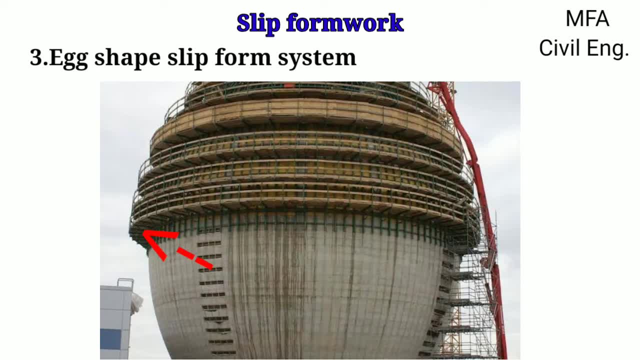 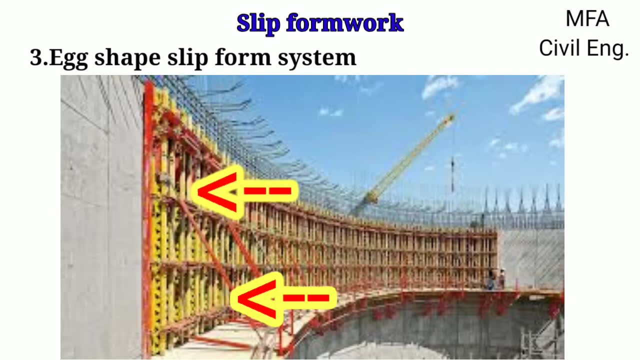 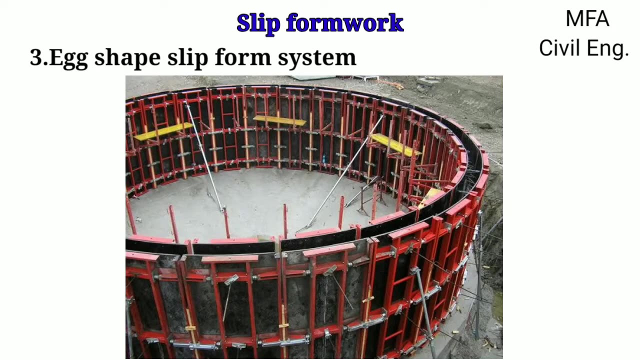 varies. the cantilever plates on the periphery are removed or extended, and the individual curvature adjustment can be achieved by adjusting the spindle and the vertical peripheral slope. both the sides of the formworks are independent of the each other, which shows the main advantage of the egg shape sleeve form system. this system can be adjusted independently on the each side of 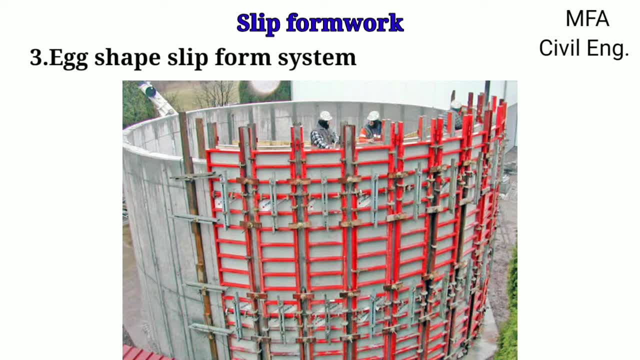 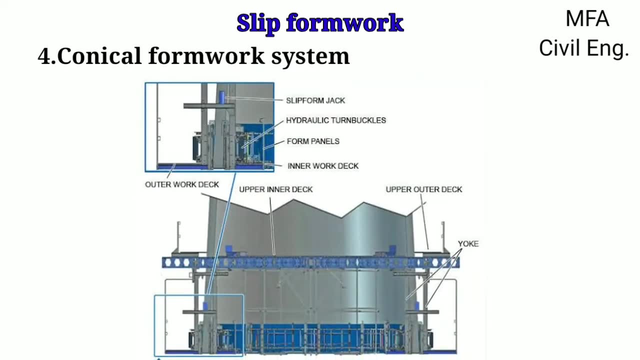 the wall and also produce a optimum working condition. it shows an apparent saving in the time and the personal cost. conical formwork is a system by which it is made possible to construct the structures of a varying wall thickness and the tapering wall. it is also possible.